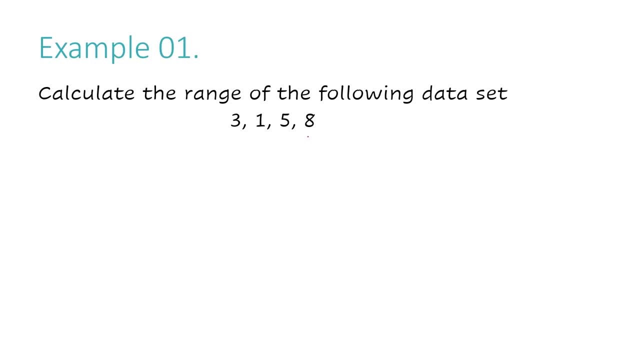 steps that I explained to you before. The first step is to identify the largest number in the data set, and in this case it's going to be eight. The second step is to identify the smallest number in your data set, and in this case it's going to be one. The final step is to subtract the two. 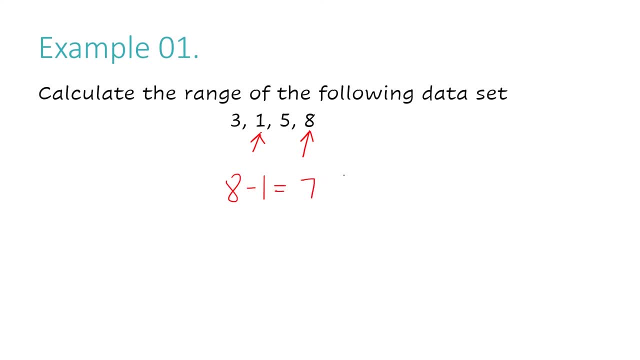 I have eight minus one, and that gives me seven. The range of this data set is seven. Let's move on to example number two. Example number two: calculate the range of the following data set. Well, my largest number is 33.. My smallest number is nine. I need to subtract these two. 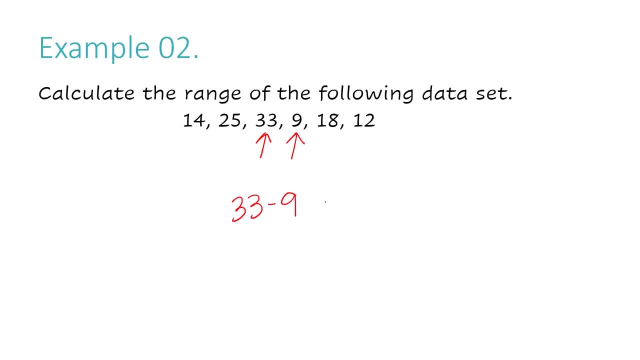 The largest number goes first, the smallest number goes second. and when I subtract, I get my answer, and my answer is the range. Whenever I have a number and it's nine and I'm subtracting something by nine, I like to round and so I say: well, let's say I took the number 33. 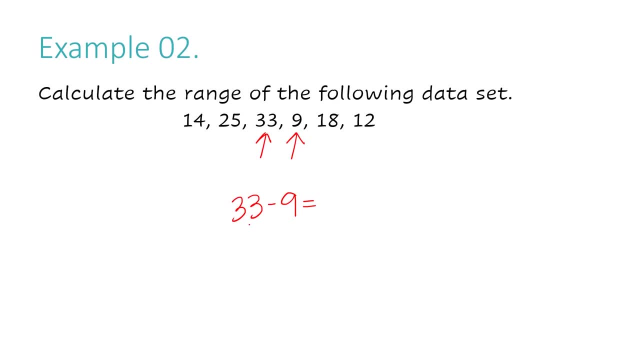 and I subtracted 10 from it. Well, I know that would give me 23,, but I didn't really need to subtract 10.. I only need to subtract nine. so I know that 23 was a little bit off, It's not. 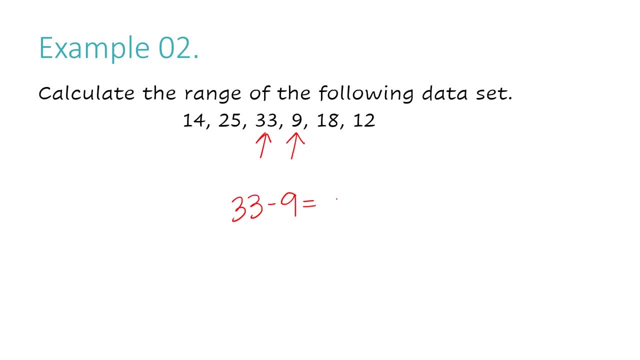 actually the correct answer, so I'm going to actually add one to it, and I know my answer's 24.. So that's how I subtract nine in my head. So the answer to example number two is: your range is 24.. So what does that mean? Do you understand what that means or are you just doing it because 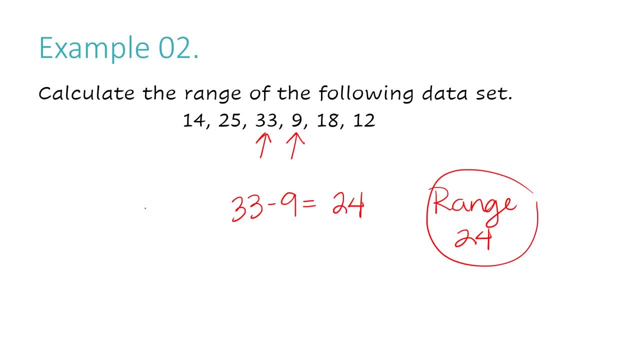 somebody told you that's how you calculate range. Let me show you what it means. It means if you have a number line, and let's say my number line is marked off in intervals of 10,, so this is 10,, this is 20,, this is 30, and let's do halfway marks, So this would be 20,. 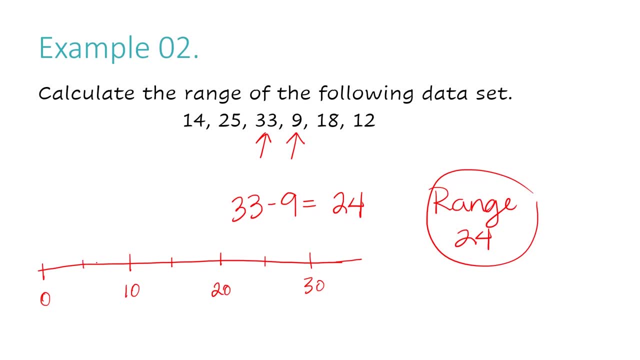 25,. this would be 15, and this would be 5.. Let's say I have all of these numbers marked off on this number line. okay, 14, that's going to fall in between here. so this is 10,, so this would be 11,. 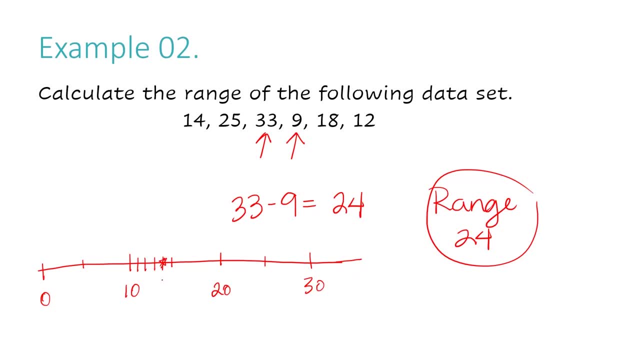 12,, 13,, 14.. This is the 14 mark. I'm going to mark it. Cross this off because I've used it. 25, that's going to be here. Cross it off because I've used it. Oh, and let me put a star. 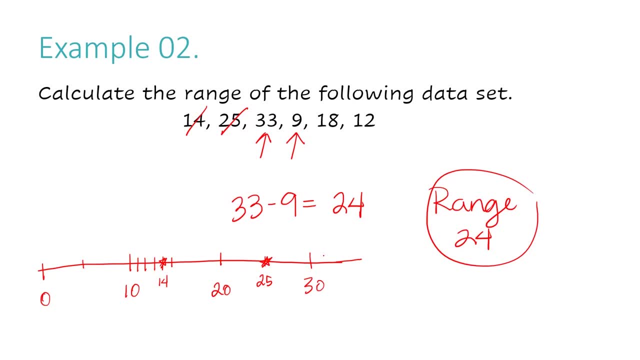 like I did the other one: 33,, 33,, 31,, 32,, 33,. put a star 9 would be 1 over. put a star 18 would be 2 to the left of the 20.. 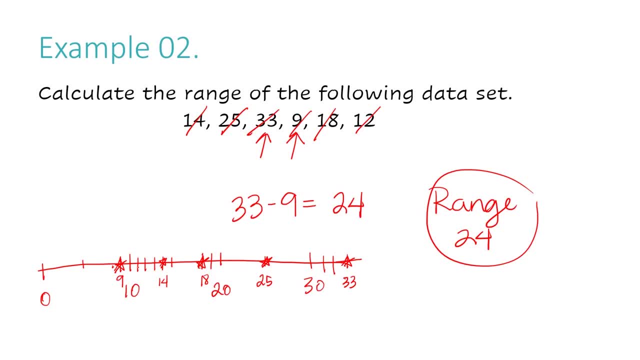 And 12 would be 10,, 11,, 12, right here. Okay. so now all of these numbers that are in my data set are listed on this number line. I'm going to go ahead and fill in these other notches. I guess I could have did that in the. 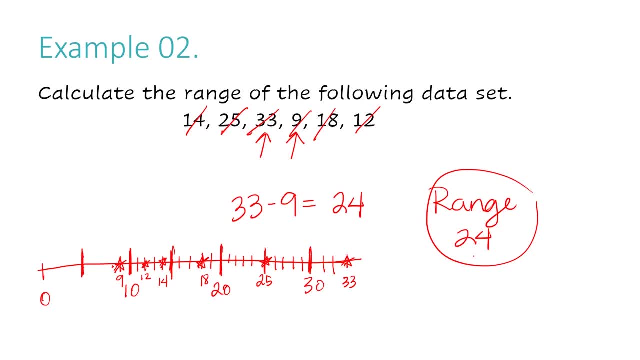 beginning to make it a little more clear, but it'll be all right. The range being 24 means the distance on the number line from my smallest number to my largest number is 24 notches. So let's count this. This is- I'm starting here- at the 9.. This is 1.. Well, this is the first space. 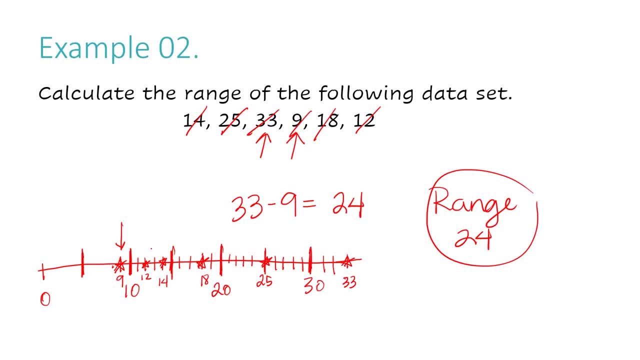 and the next one over is 1,, 2,, 3,, 4,, 5,, 6,, 7,, 8,, 9,, 10,, 11,, 12,, 13,, 14,, 15,, 16,, 17,, 18,, 19,, 20,, 21,. 22,, 23, 24.. Okay, get that distance raise from with them. Oh, put a star 42,, 23,, 24,, 22.. And I'll do this. next one will is 1.1, 2,, 3.4,, 5,, 6,, 7,, 8,, 9,, 10,, 11,, 12,, 13,, 14,, 15.. 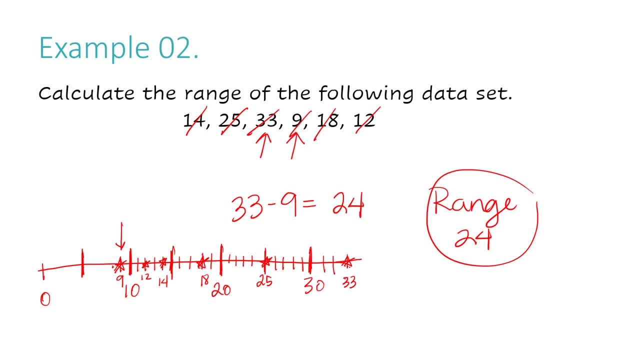 64,. So if I were to go along my number line, starting at the smallest number in my data set and ending at the largest number in my data set, I would have moved 24 spaces over my number line. that's what your range is. okay, so when we're calculating the range, we're 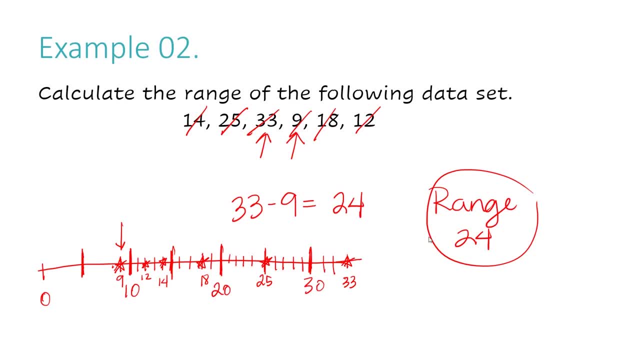 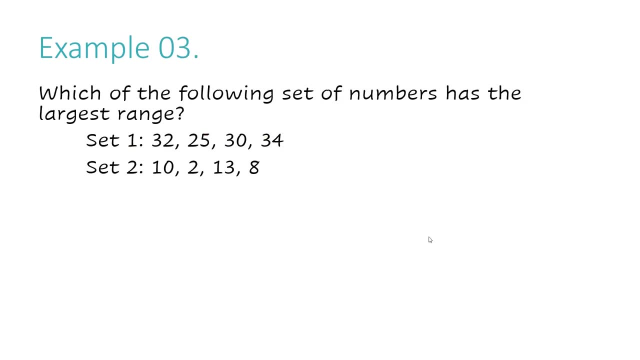 trying to figure out how many spaces does this data set take up on a number line. let's look at example number three. which of the following data sets of numbers has the largest range? okay, so this takes it a step further. we're going to calculate the range twice, for two separate data. 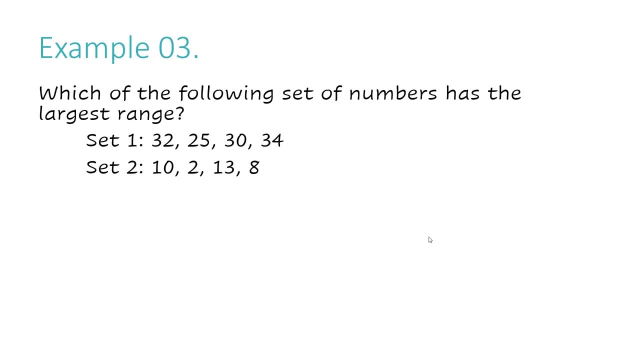 sets and then we just answer the question: which set has the largest range. so for my first set I gotta figure out my smallest number and my largest number and subtract: my smallest is 25, my largest is 34. I subtract them so I have 34 is the largest, minus the 25, and that would give me 9. 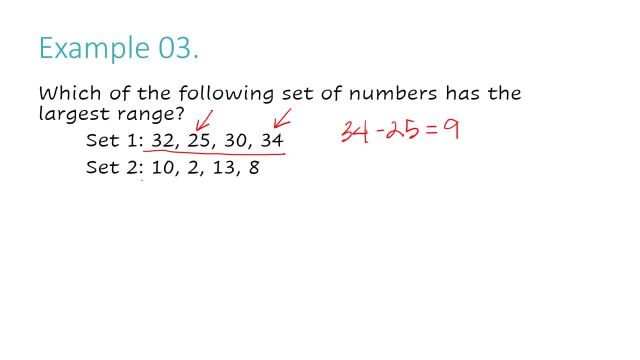 the range of data set one is 9. I got to figure out my range and then I keep on going the minimum range. I guess it's something that's just a lot to do. range of data set two: Okay, my largest is 13.. My smallest is two. So I subtract those 13 minus two. 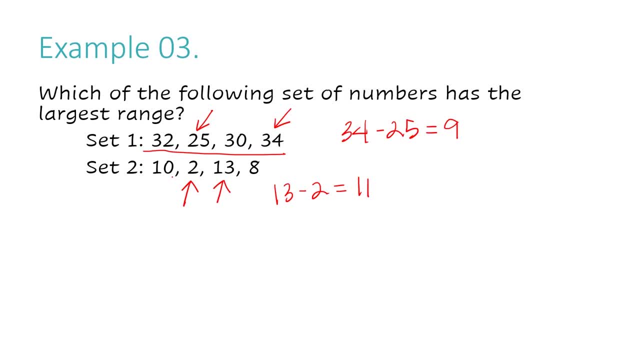 equals 11.. My range for data set two is 11.. Do not think: oh well, the numbers in data set one are larger numbers, So that means it's going to have the larger range. No, that's not necessarily true. In this case, you can see that this has a larger range. That means this has a longer space. 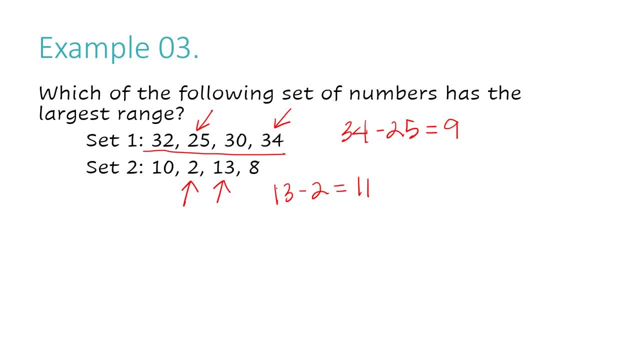 that it takes up. on the number line, It goes across 11 notches. on the number line, The first data set would only go across nine notches. Okay, when I'm answering the question of which of the following data sets has the largest range that would be set two. 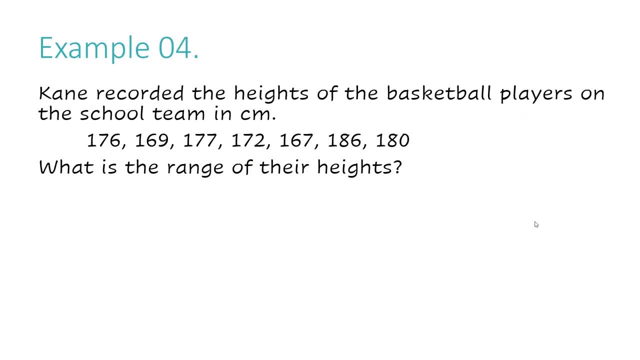 Let's take a look at example number four. Kane recorded the heights of the basketball players on the school team in centimeters. What is the range of their heights? Well, I need to find the largest and I need to find the smallest and I need to subtract them. I got 176, 169, 177, 172, 167,. 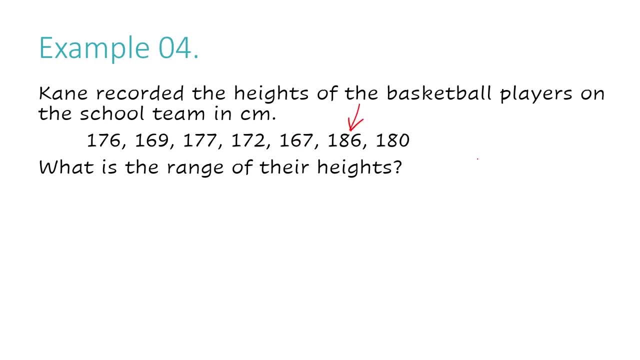 186, and 180.. Okay, 186,, that's my highest. My smallest looks like it is the 167.. Minus 167.. So if you were going to manually subtract this, you could take the 186,, stack it. 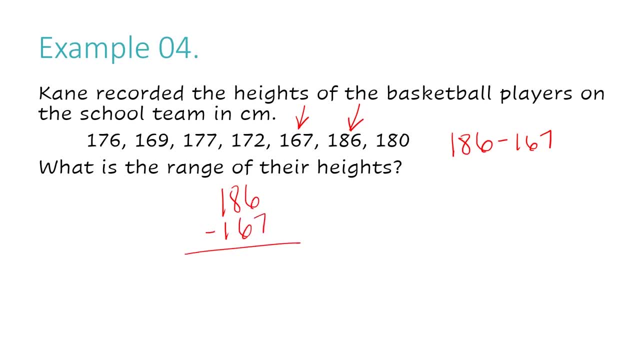 on top of 167.. And remember, you're gonna have to make that a 16, make this one less, because you're borrowing or regrouping. 16 minus 7 is 9.. And then here's a 1, and that's just 0.. So the difference. 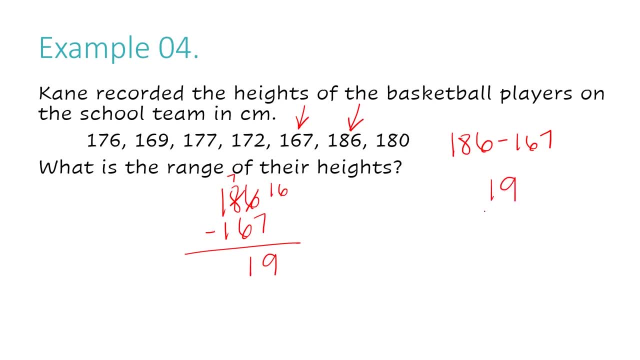 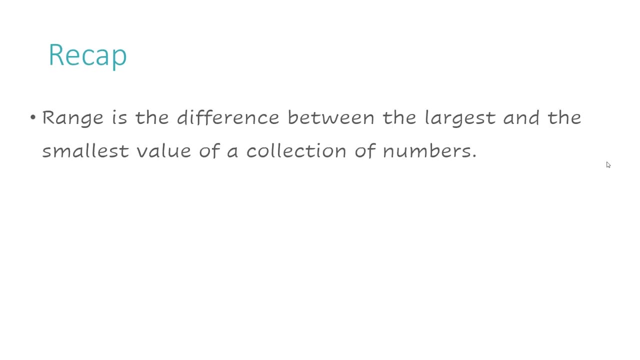 between the two is 19.. So what's the range of the height of the basketball players on the school team? The range of their heights, 19.. And remember these were centimeters. So you want to say that the range is 19 centimeters. Now let's take a recap Recap. The range is the difference between: